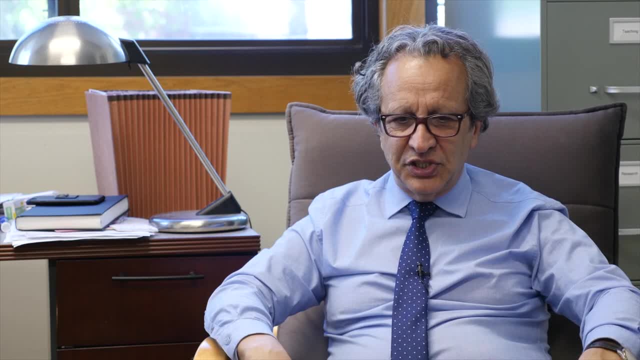 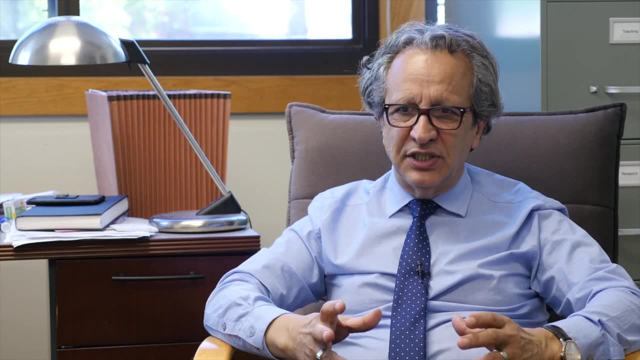 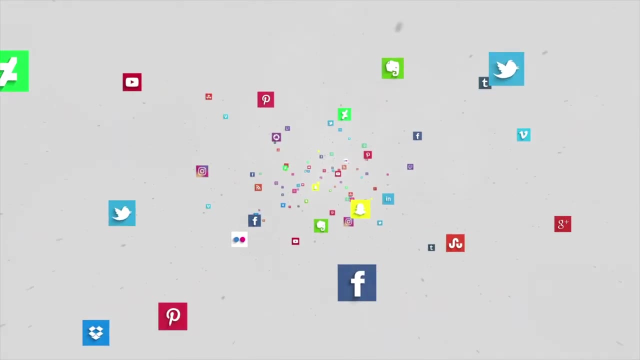 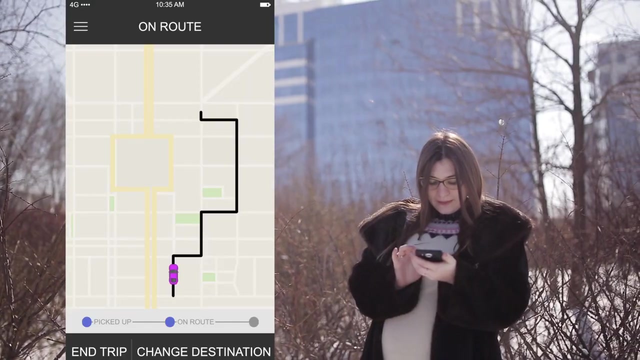 The reason HCI is important in understanding the real role and place of technology in our societies is that technology is not just objects and artifacts. Technology is much more than that And HCI essentially, among other things, provides that broad perspective in terms of what it means to people, how it changes and shapes our ways of life. 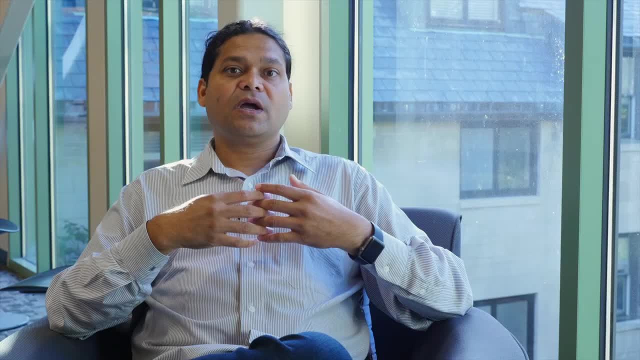 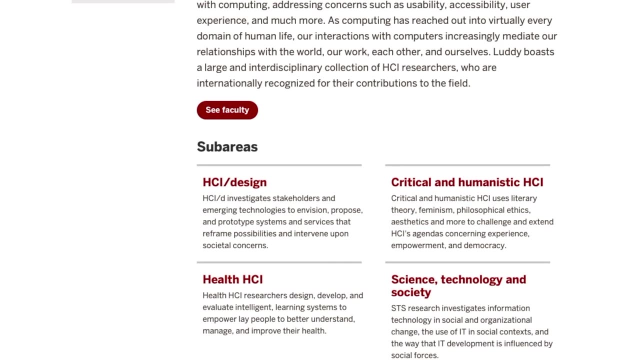 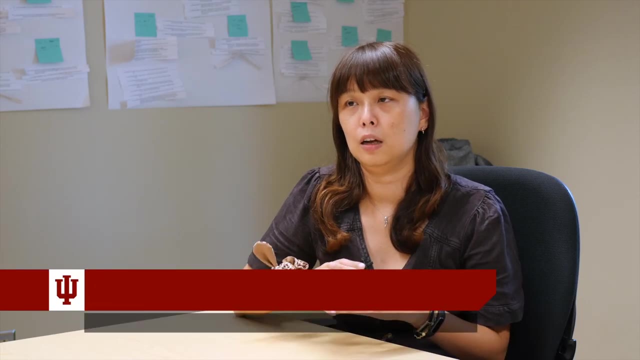 We are living in the golden age of HCI research right now. In HCI we have faculty across our departments, not just within informatics but across in computers science, as well as an engineering, information library science, who are working on HCI problems. We have like an extensive number of like health HCI researchers. we have some of the best design. 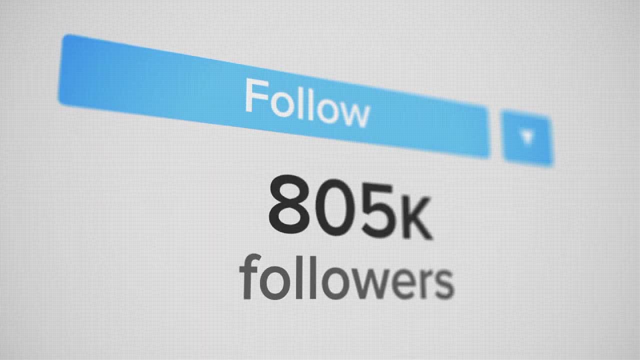 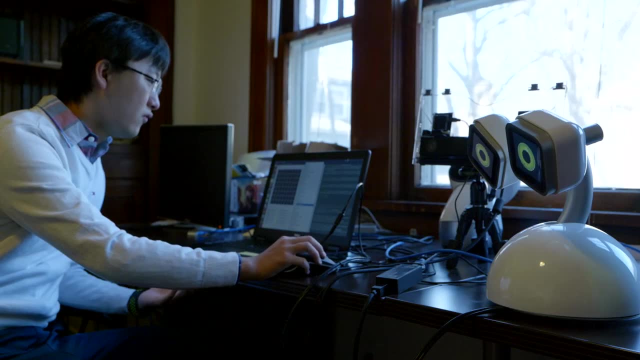 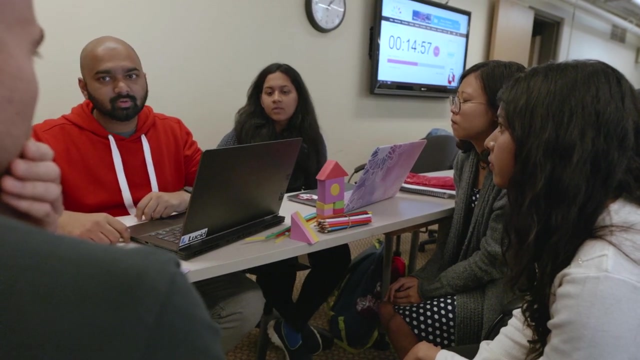 researchers in the field. we have people understand the society impact. we have people do privacy and robotics and different ways that people can interact with technology, By bringing in a whole bunch of people from different backgrounds, different areas, different countries, different perspectives to try to solve problems together. that's when we 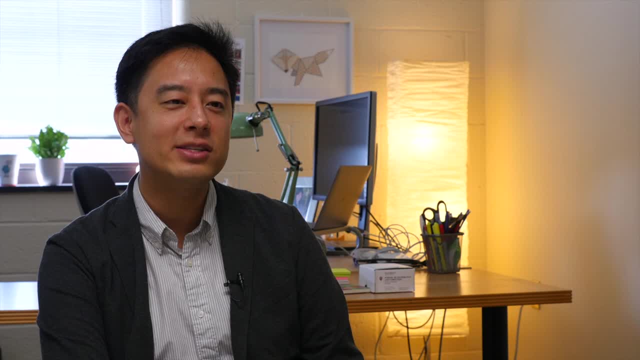 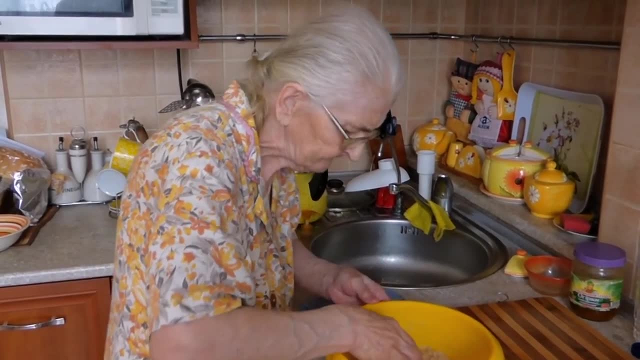 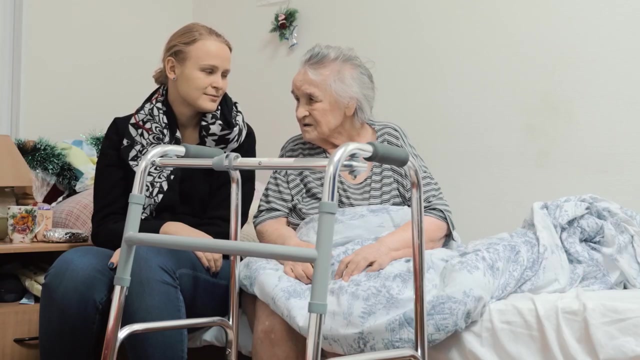 learn the most from each other. I think it's an overall theme also in HCI and in our department also is thinking about these more. you know some ignored populations or marginalized populations. If you have an interest in changing the lives of the left behind populations and making an impact that way, there's no better place to do it. 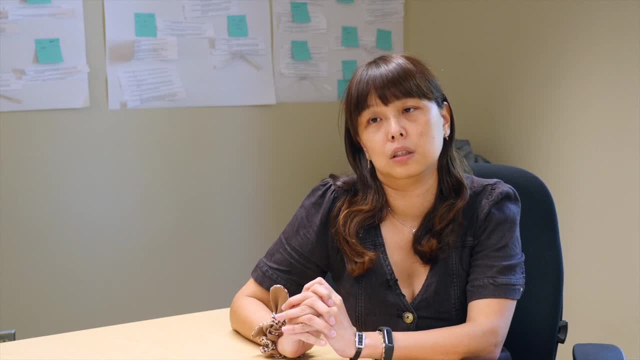 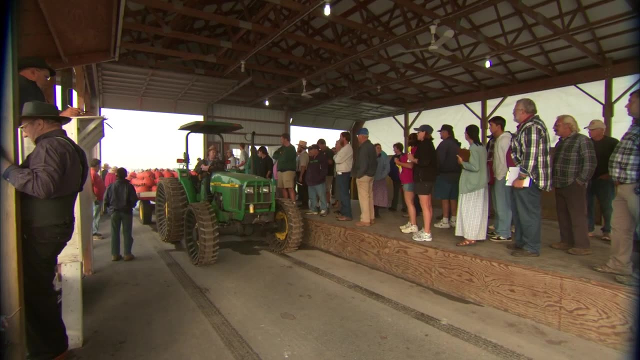 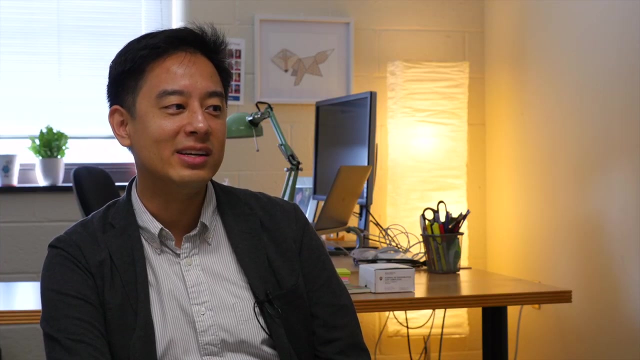 I think in Indiana we have very unique opportunities. The research that we are conducting has a direct reach to these people in rural communities and they can reach the max impact because they are the people who needed this kind of solution the most. In a lot of research I do, I study, you know different. 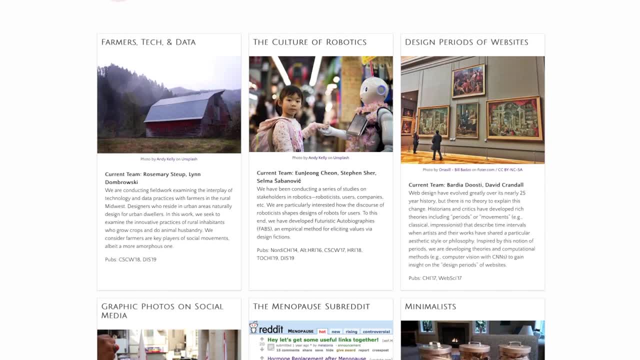 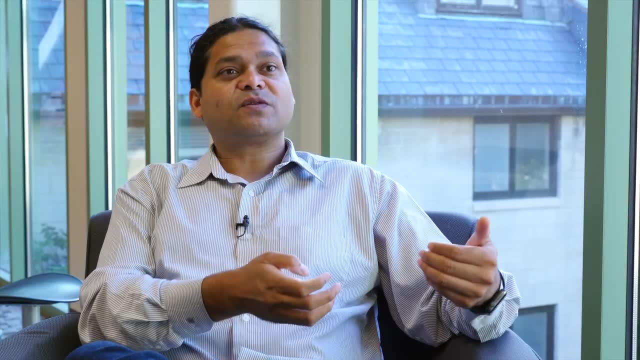 subcultures. how's it changing the traditions they're used to? right Technology might be disrupting their way of life. If the model with which the systems are built comes from the western world, that may not necessarily fit how they're used outside of the western world. So that's why we need 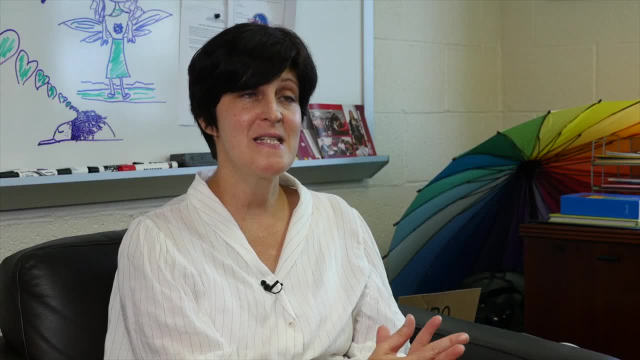 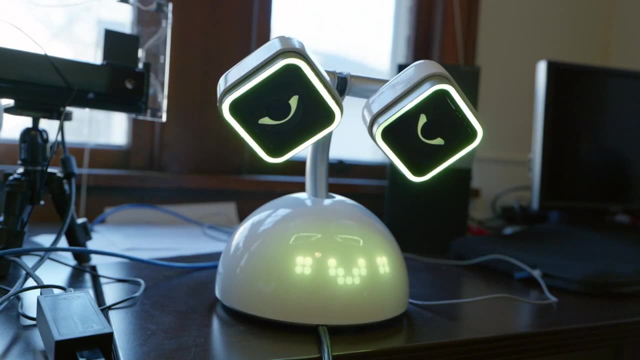 research that looks at all of these things. The research questions in a sense are endless, because I think both human computer interaction and human robot interaction are fields that are trying to invent the future. as they go along, The research at IU is going to be very progressive.